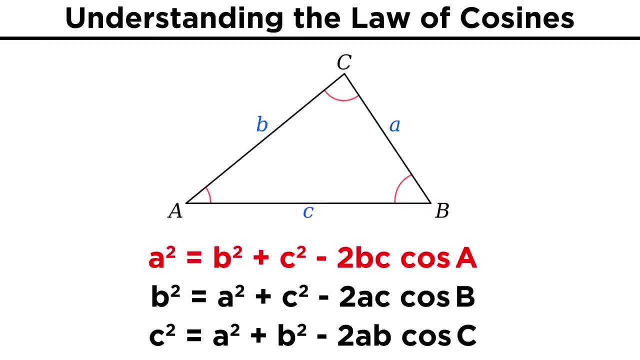 A squared equals B squared plus C squared minus C squared, Minus two B, C cosine A. As you can see, the square of the missing length is expressed in terms of the other two lengths and the angle between them, While the law of sines allowed us to solve side angle, angle, angle, side angle and side. 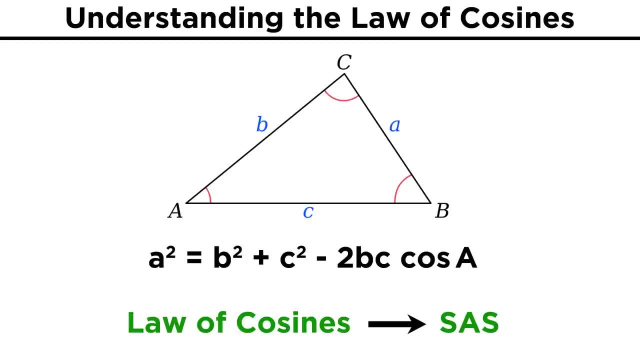 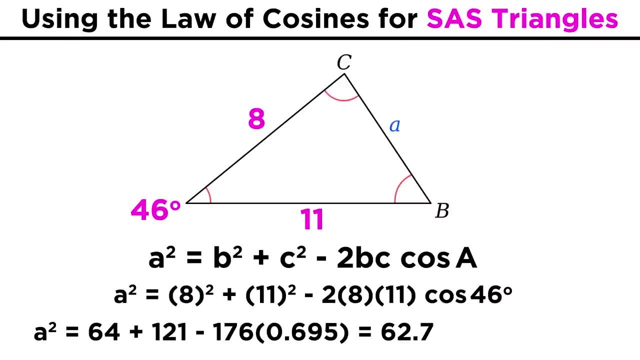 side angle triangles. now, with the law of cosines we can solve side angle side triangles. Take this one, for example. We've got our two sides and the angle between them known. So let's plug everything into the equation, Simplify a little bit, and there's our value for the third side. 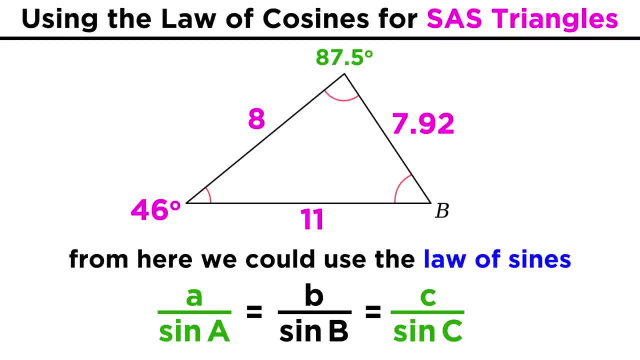 From here we could use the law of sines to get one more angle, and then subtract these two from one eighty to get the final angle. Now we know everything about this triangle. Notice that we couldn't have solved this with the law of sines alone. 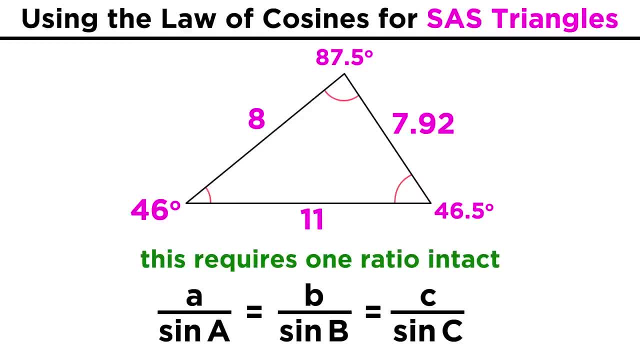 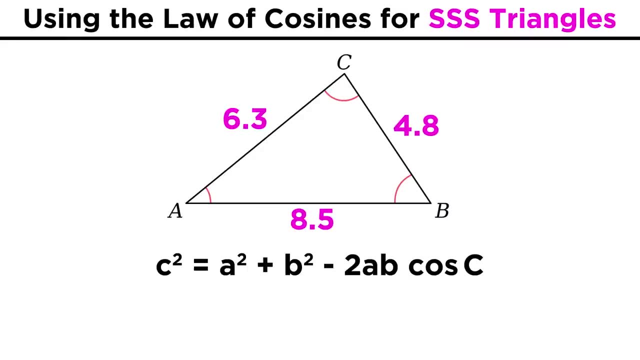 Because to use that law, we need one side and angle that correspond to one another, as well as one other piece of information in order to start using the ratio. With the law of cosines, we can also solve for side, side, side triangles. 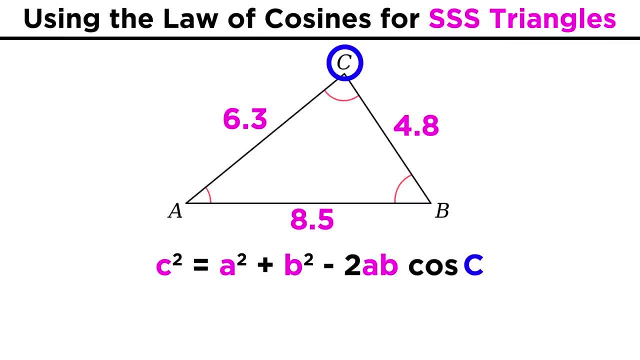 This is because if we know all three side lengths, we can solve for any one of the angles. The easiest way to do this is to solve for the angle that is opposite the longest side. So let's do that. So for this triangle, let's call the longest side C, Using the general formula. let's: 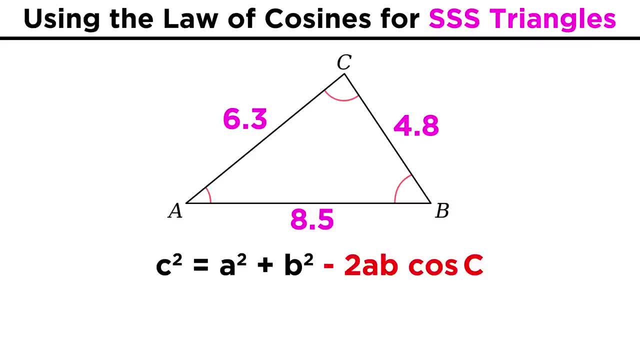 solve for angle C. Bring this term containing the angle to the other side and make it positive and bring C squared to the other side. Then we just divide and now we are ready to plug in all the values. We plug in side lengths A, B and C. 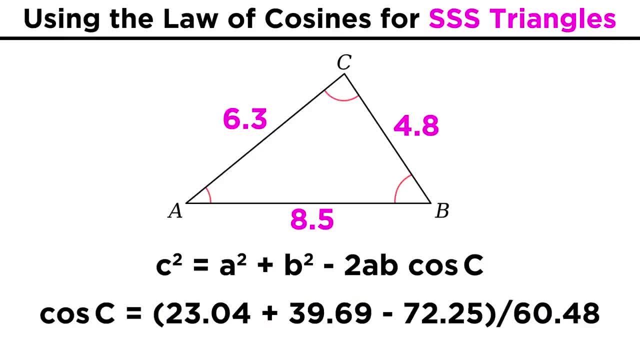 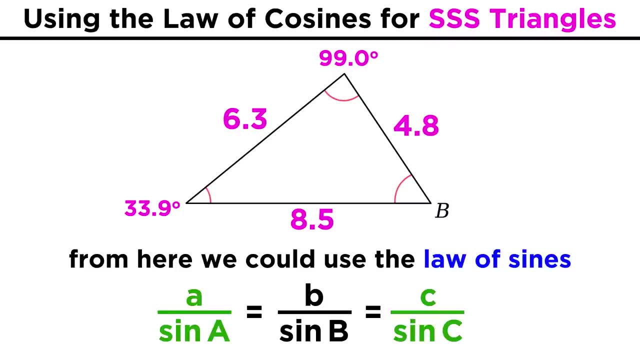 Simplify and we get our answer. for cosine of C, We take the inverse cosine and there's our angle to the nearest tenth From here. we just use the law of sines to get one more angle and then subtract these.